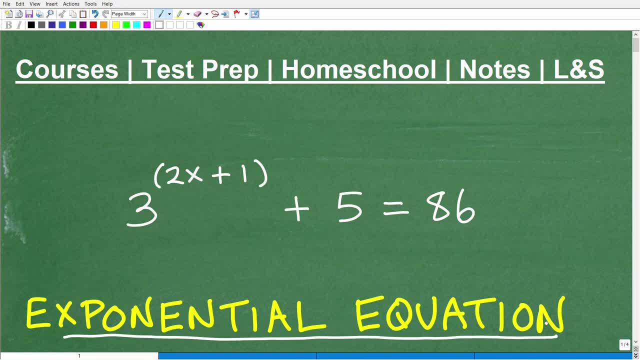 Maybe intermediate algebra. So if you happen to be taking pre-algebra or even algebra one, you may not have seen everything I'm going to be talking about in this particular video, But do not run away, as you will learn the basics of solving an exponential equation. Now, this is really really important stuff in algebra and it's not that difficult. But anyways, before we get going, let me quickly introduce myself. My name is John. I'm the founder of TC Math Academy. I'm also a middle 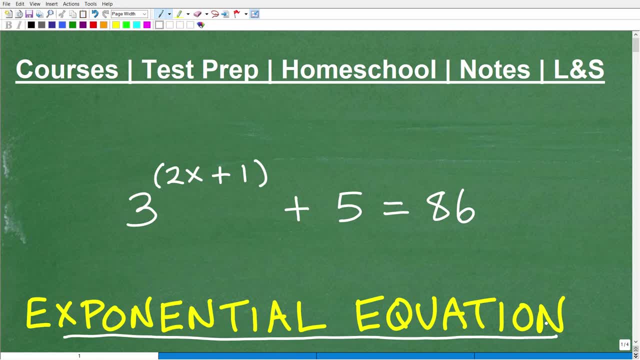 and high school math teacher. I have been teaching math for decades. It really is my true passion to help as many people as I possibly can learn mathematics. And I'm going to tell you right now: all of you can be successful in math, And I'm especially speaking to those of you that have a difficult time in mathematics. Please do not give up. There's absolute hope for you not to only just pass your math class if you happen to be taking a math course, but for you to excel in math. But here's the thing you need: You need great math. 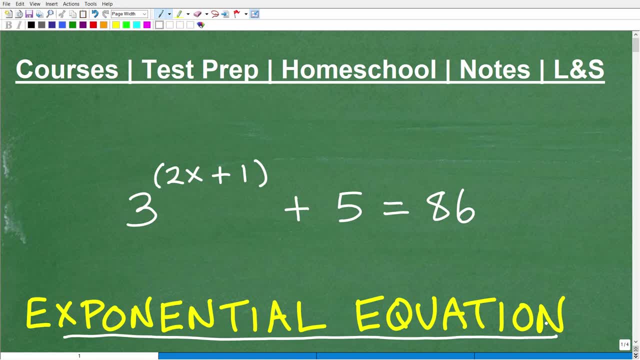 Math instruction, ie whoever you're learning from, or whatever you're learning from. If you're confused and you're not understanding what the teacher is teaching you, you are not learning. Now, that seems pretty obvious, but you have to find instruction that you understand. In other words, when you're being taught something, you actually get what's going on. Now, math is a technical subject and the way I like to teach it is to kind of demystify things and make it kind of easy to understand for everybody, without watering down what you need to know. 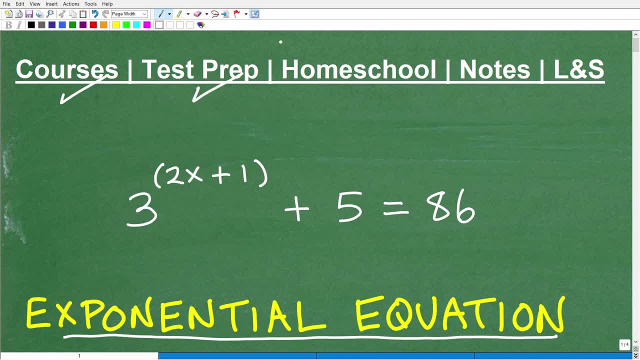 So if you need help in your current math course or maybe some sort of special test that you're getting ready for that has math on it- I'm talking about things like the SAT, GED, maybe a teacher certification exam- Or if you're homeschooling mathematics, check out my math help program. I'm going to leave a link to it in the description of this video. I literally have over 100 plus different math courses that span these categories and much, much more. I'm also going to leave links to my math notes in the description as well. If you truly want to be great at math, you must take great math. 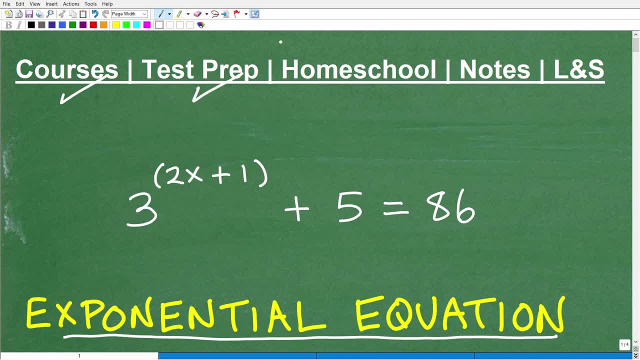 So if you need help in your current math course or maybe some sort of special test that you're getting ready for that has math on it- I'm talking about things like the SAT, GED, maybe a teacher certification exam- Or if you're homeschooling mathematics, check out my math help program. I'm going to leave a link to it in the description of this video. I literally have over 100 plus different math courses that span these categories and much, much more. I'm also going to leave links to my math notes in the description as well. If you truly want to be great at math, you must take great math lessons. 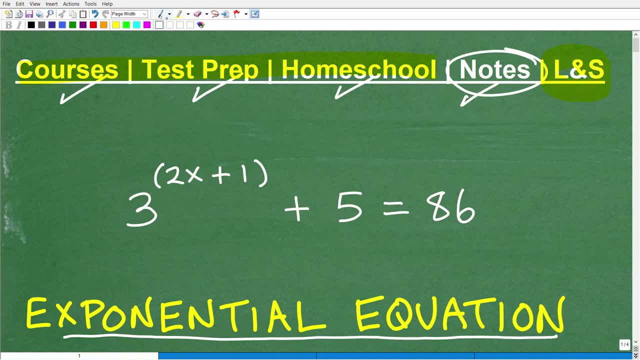 This is so, so important, And if this video helps you out, don't forget to like and subscribe, as that definitely helps me out. Okay, so let's go ahead and take a look at the solution for this particular video. Again, we are talking about exponential equations. Now let's just go ahead and just real quick talk about this term here: exponential equation. Obviously, this is an equation, but the variable that we're trying to solve for x is located in the exponent position, in particular. 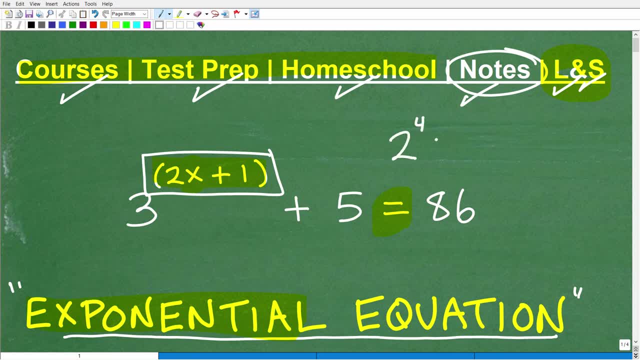 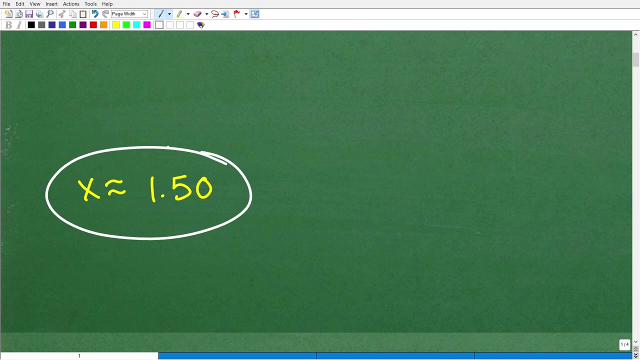 In terms of this power, right? So if you have like two to the fourth power, of course, that's 16.. Two is the base, four is the exponent, and then this would be the answer. So this location up here is the exponent. The variable is in the exponent. That's why we call this an exponential equation- Big, big topic. But let's go ahead and take a look at the answer for this particular equation. right now It is approximately 1.50.. So that's what x would be equal to, approximately 1.50.. I am rounding off a. 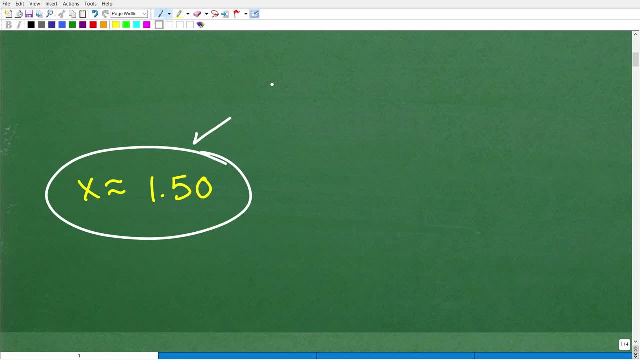 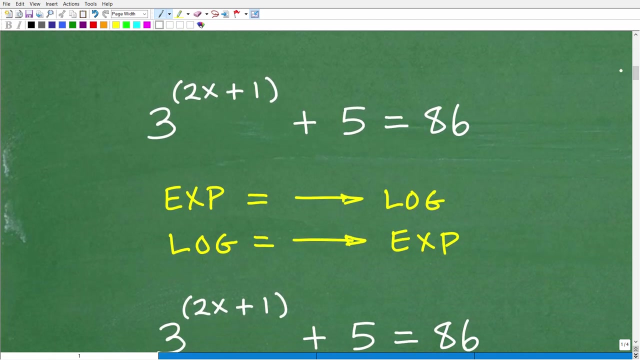 bit, But if you happen to get this correct, that's very impressive. Matter of fact, I'm definitely going to reward you with a nice little happy face and a plus a 100% and a few stars, So you could tell your friends and family that you know how to solve a basic exponential equation. All right, so let's go ahead and get into this right now. Now again, I already kind of told you why this is an exponential equation, But here's the main thing you need to know. So when you have an exponential 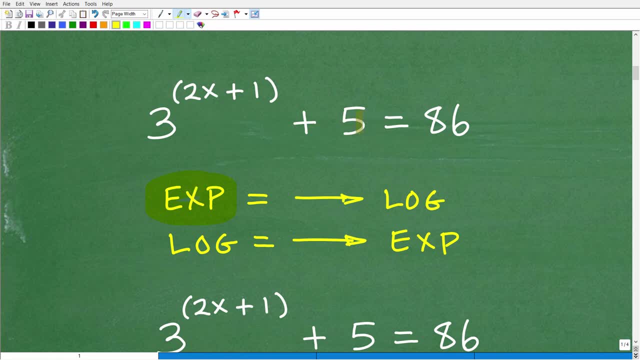 equation. as you know our particular problem right here. you need to solve it using logarithms. Okay now, if you've never seen a logarithms before, if you look on your scientific calculator or graphing calculator, it's this button. right here It's log. you'll see this button and you'll see. 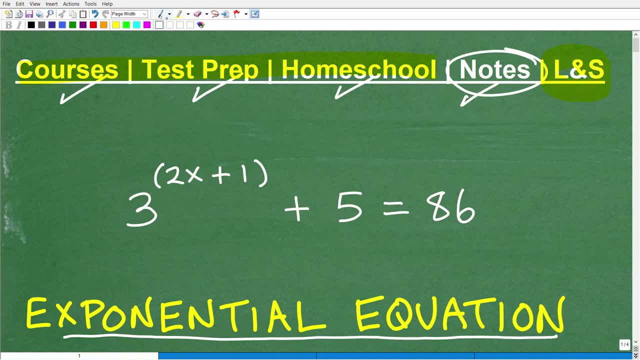 math notes. This is so, so important, And if this video helps you out, don't forget to like and subscribe, as that definitely helps me out. Okay, so let's go and take a look at the solution for this particular video. Again, we are talking about exponential equations. Now let's just go ahead and just real quick talk about this term here: exponential equation. Obviously, this is an equation, but the variable that we're trying to solve for x is located in the exponent position in 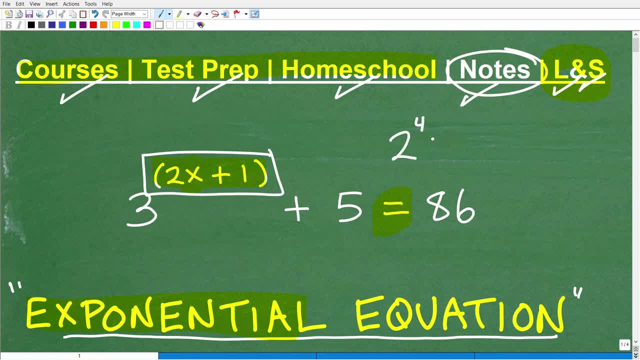 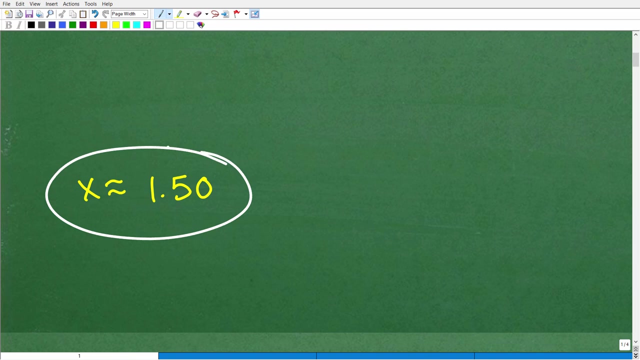 terms of this power, right? So if you have like two to the fourth power, of course that's 16.. Two is the base, four is the exponent, and then this would be the answer. So this location up here is the exponent. the variable is in the exponent. That's why we call this an exponential equation- Big, big topic. But let's go ahead and take a look at the answer for this particular equation. right now. It is approximately 1.50.. So that's what x would be equal to: approximately 1.50.. I am rounding off. 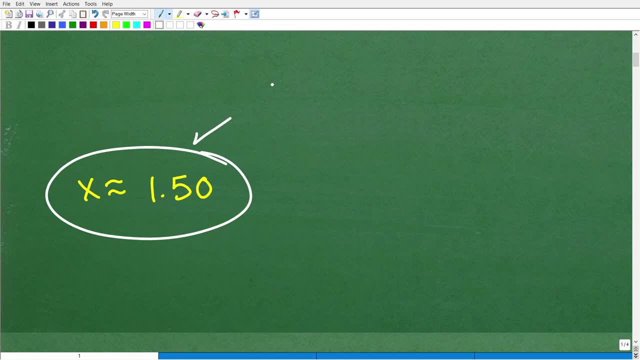 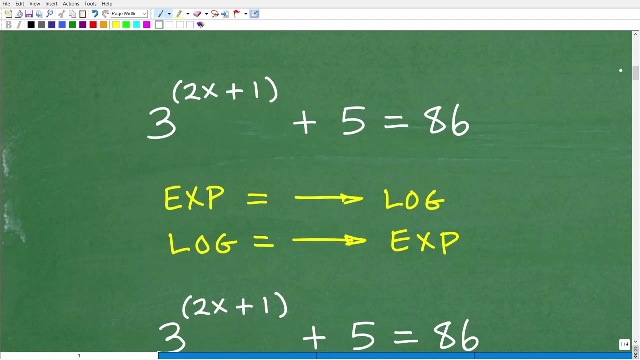 a bit, But if you happen to get this correct, that's very impressive. Matter of fact, I'm definitely going to reward you with a nice little happy face and a plus a 100% and a few stars, So you could tell your friends and family that you know how to solve a basic exponential equation. All right, so let's go ahead and get into this right now. Now again, I already kind of told you why this is an exponential equation, But here's the main thing you need to know. So when you have an exponential 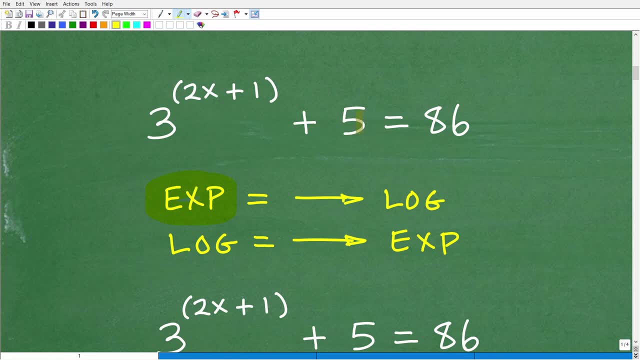 equation. as you know our particular problem right here. you need to solve it using logarithms. Okay now, if you've never seen a logarithms before, if you look on your scientific calculator or graphing calculator, it's this button. right here It's log. you'll see this button and you'll 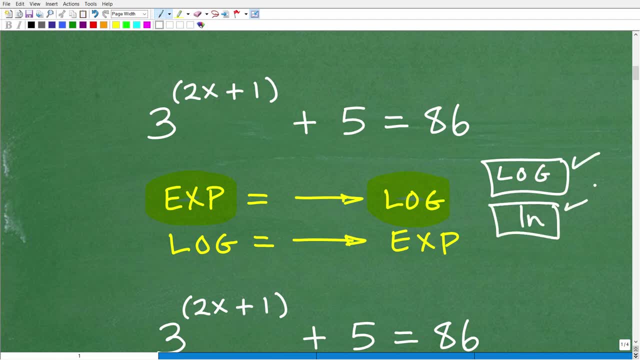 see another button L, and these right here are what we call logarithms. Now, if you've never used logarithms before, they are awesome And they're absolutely critical When you learn more advanced mathematics. but here's the main idea, right? I'm looking at this equation. I'm like 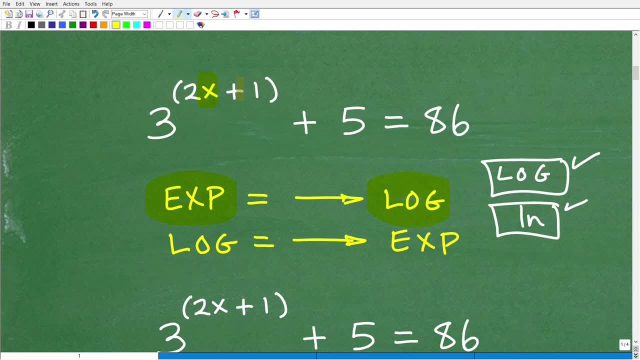 oops, I got to solve for the variable. it's in the exponent. So I'm thinking: oh, exponential equation, I'm going to have to be using logarithms. Now the reverse is true If you see a logarithmic. 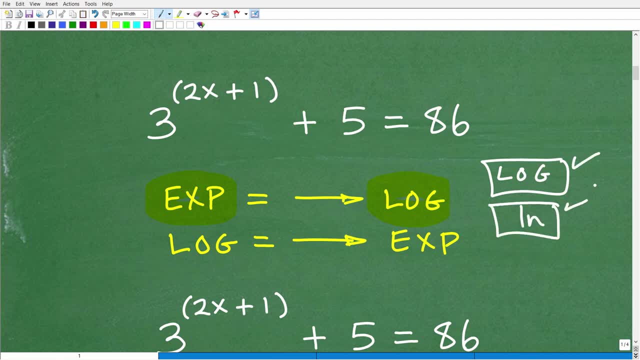 another button, L, and these right here are what we call logarithms. Now, if you've never used logarithms before, they are awesome and are absolutely critical When you learn more advanced mathematics. but here's the main idea, right? I'm looking at this equation like oops, I got to. 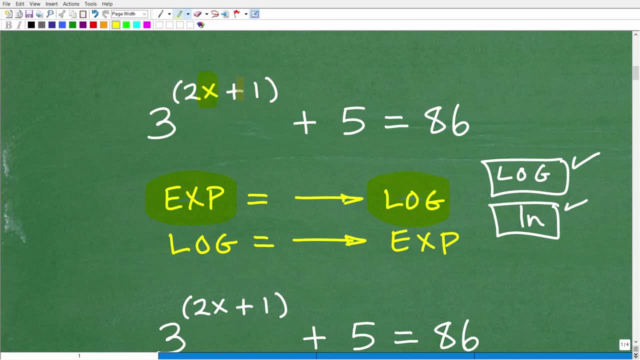 solve for the variable. it's in the exponent. So I'm thinking, oh, exponential equation, I'm going to have to be using logarithms. Now the reverse is true: If you see a logarithmic equation- of course we don't have one here- you're going to be using exponents to solve that. So the main idea: 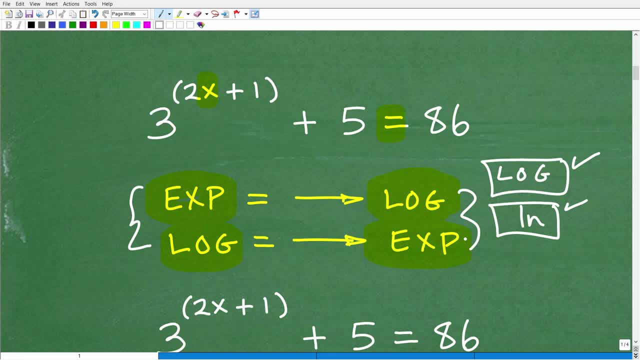 before we get started, is that exponential functions and logarithmic functions are inverses of one another. Okay, so kind of keep that big picture in mind. you'll be able to solve both exponential and logarithmic equations. Now, of course, because we have an exponential, 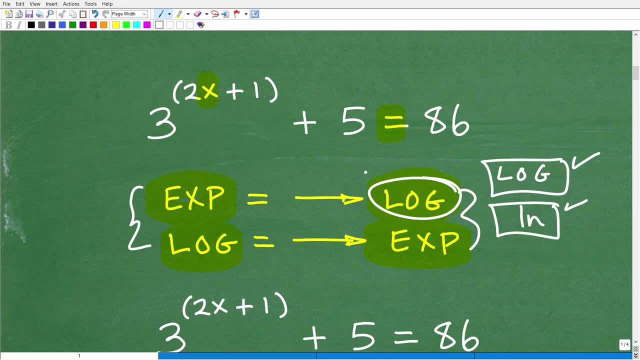 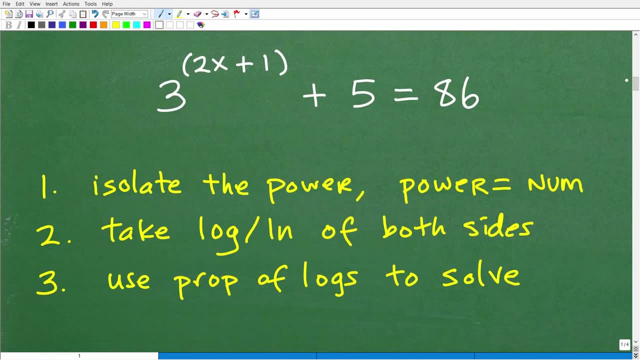 equation, you're going to need to know something about logarithms And I'll kind of explain some basic stuff here in a second. All right, so kind of getting that out of the way. in terms of the big picture, let's look at the specific steps to solve an exponential equation And I kind of just 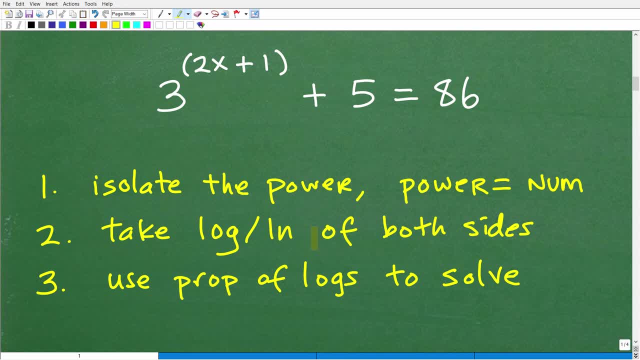 pretty simple And using easy language here. you know I can make this more detailed, but I think this is good enough. So the first thing is: you want to isolate the power. Okay, now, what am I talking about? Well, I'm talking about this part of the equation, right? So we want to get this. 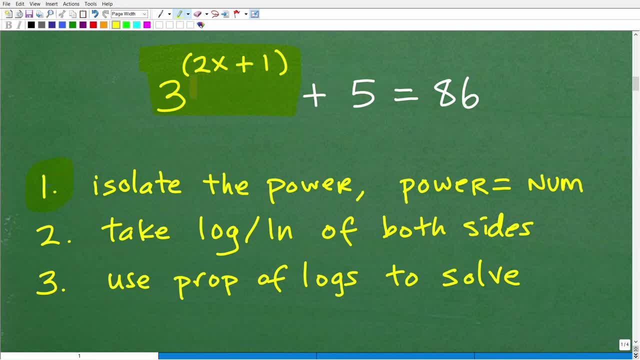 power. Now we have this power plus five. sometimes you have other things going on as well, But you want to isolate the power all by itself And effectively. what you want to do is to manipulate the equation such that you have the power on one side, like the left hand side. 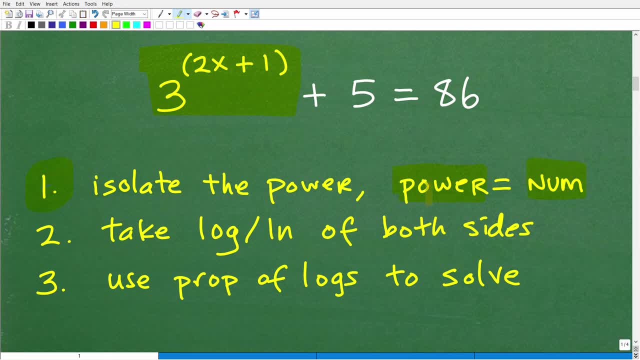 and you have a number on the other side. So you're going to have to do some algebra to get to that stage. That's your first kind of series of steps that you need to do when we're solving an exponential equation. All right so, but once we got it down to this, what we're going to? 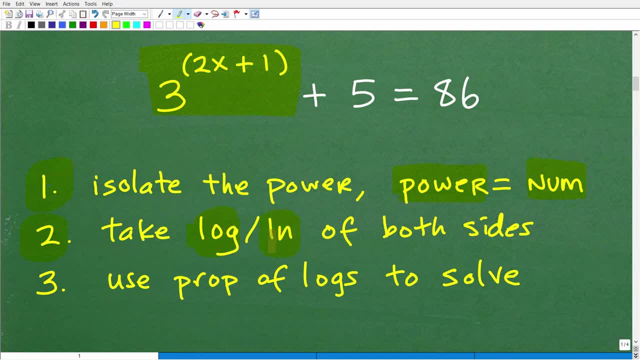 do is take the log or the ln. that's ln, not in, that's the. basically, both of these are logarithms. we're going to take the log of both sides. Now let me just tell you real quickly here, because a lot of you probably don't know this, but we're going to take the log of both sides. 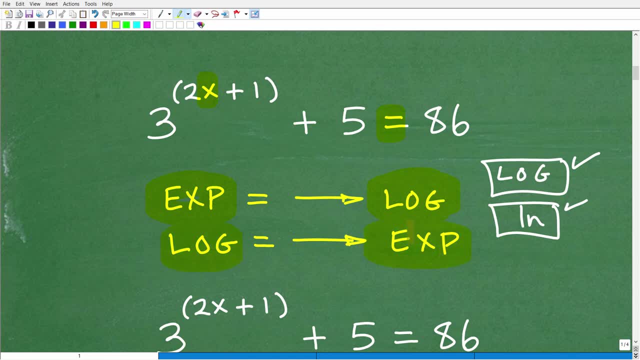 equation. of course we don't have one here. you're going to be using exponents to solve that. So the main idea before we get started, is that exponential functions and logarithmic functions are inverses of one another. Okay, so kind of keep that big picture in mind, you'll be able to. 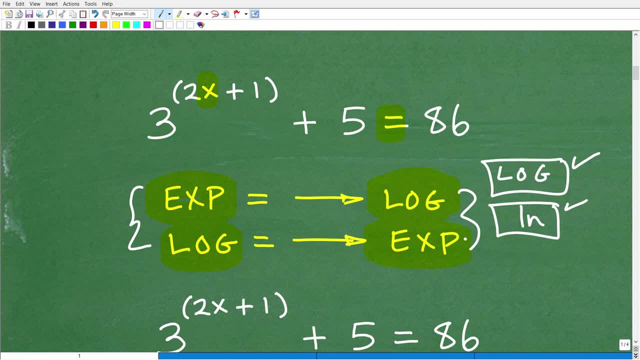 solve both exponential and logarithmic equations. Now, of course, because we have an exponential equation, you're going to need to know something about logarithms, And I'll kind of explain some basic stuff here in a second. All right, so kind of getting that out of the way. in terms of the 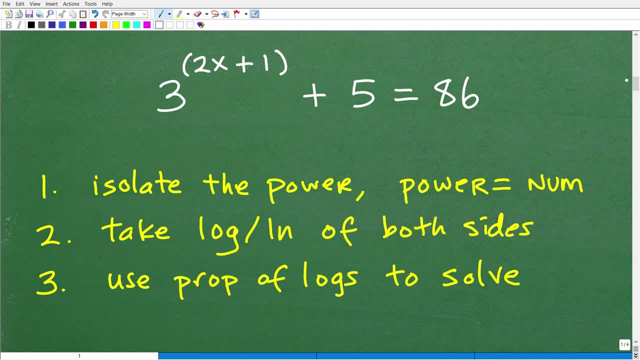 big picture. let's look at the specific steps to solve an exponential equation. And I kind of just pretty simple and using easy language here. you know I can make this more detailed, but I think this is good enough. So the first thing is you want to isolate the power. Okay, now what am I? 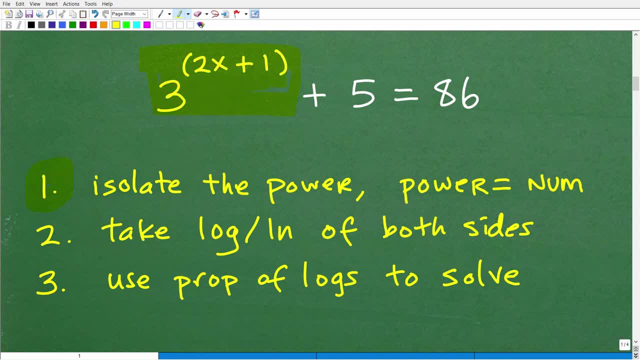 talking about? Well, I'm talking about this part of the equation, All right. so we want to get this power Now, we have this power plus five. sometimes you have other things going on as well, But you want to isolate the power all by itself And effectively. what you want to do is to manipulate. 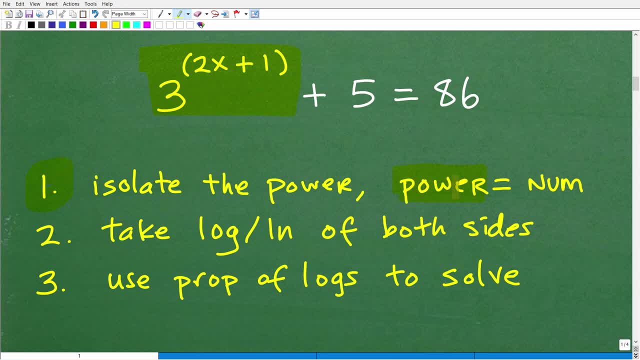 the equation such that you have the power on one side, like the left hand side, and you have a number on the other side. So you're going to have to do some algebra to get to that stage. That's your first kind of series of steps that you need to do when we're solving. 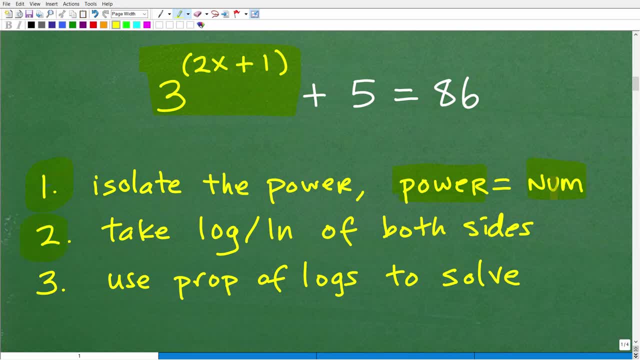 an exponential equation. All right so, but once we got it down to this, what we're going to do is take the log or the ln. that's ln, not in, That's the. basically, both of these are logarithms. we're going to take the log of both sides. Now let me just tell you real quickly here. 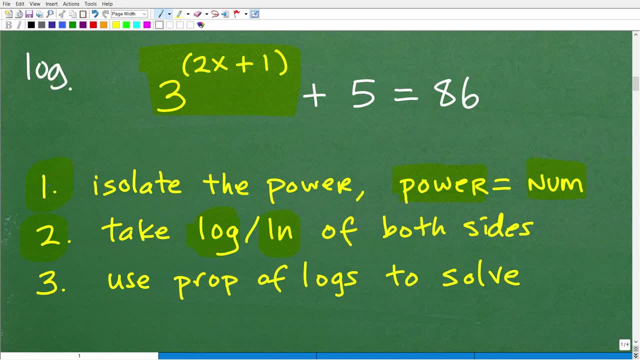 if you're probably confused, log this here is a common log. it's log base 10.. ln is what we call the natural log. it's log base e. Again, if you don't know much about logarithms, all this stuff, 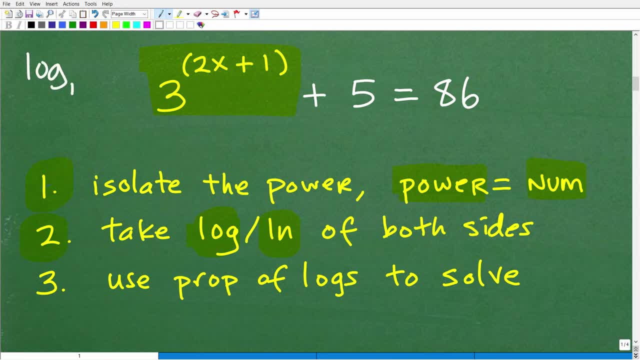 You're probably confused. Log- this here is a common log. it's log base 10.. ln is what we call the natural log. it's log base e. Again, if you don't know much about logarithms, all this stuff, 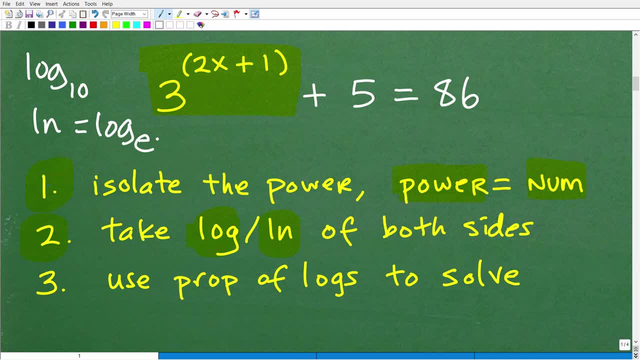 you can learn thoroughly. If you check out any one of my courses, I would recommend my algebra two course. if you happen to be in pre calculus, I teach this in that course as well, but it will not be in my algebra one course, as you don't really most students will not get it. 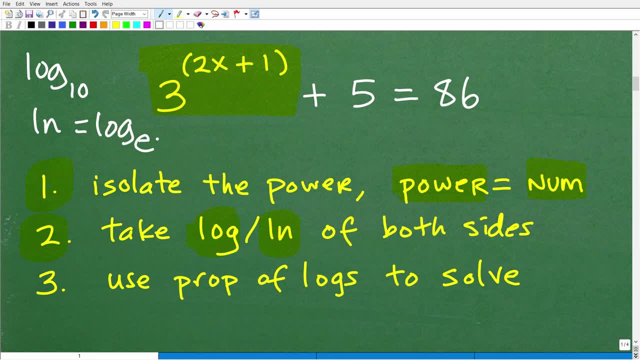 logarithms until algebra two or college algebra. Okay, so, anyways, we're going to go ahead and take the log of both sides. Now, how do you know whether you take the ln or common log? this is log base three. Now, if I had a problem like x or- sorry, e to the two, x is equal to one. this is the natural. 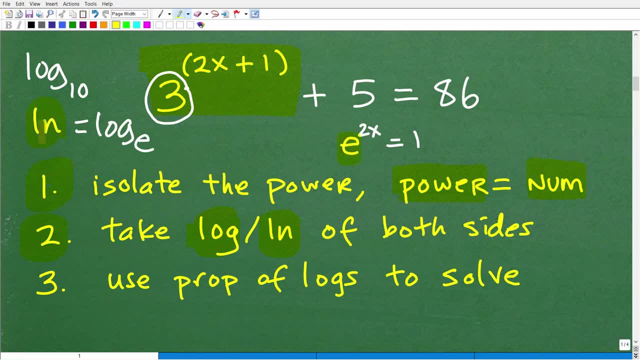 base e. So anytime you see e, you'll take the ln. okay, the natural logarithm. If you see numbers as a base, you'll take the ln. So anytime you see e, you'll take the ln. So anytime you see e, you'll take. 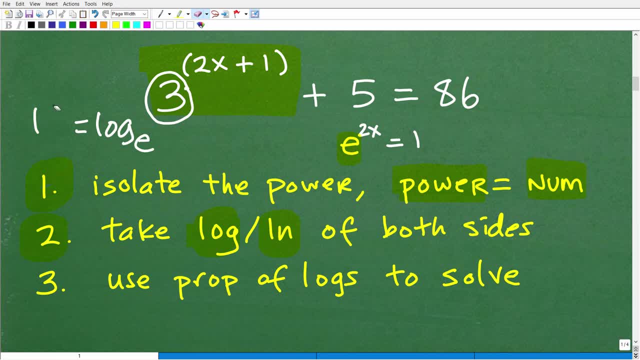 the common log. Now, if you did take the natural log you still would get the answer right, But it's just more kind of typical to just take that common log. Okay, so we're going to take the log of both sides And then, lastly, we're going to use the property of logs, or logarithms, to solve for that. 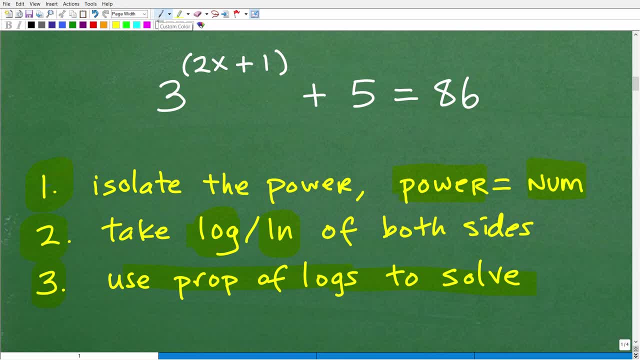 variable. All right now, if you, you know, again, haven't studied logarithms in detail, I'm going to go ahead and show you an example of these three steps, And you'll learn how to do that in just a minute. So at least get a sense of what's going on. But again, if you are taking this, this should. 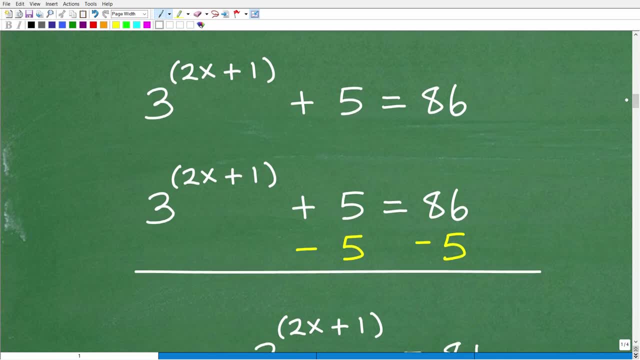 be a pretty if you're taking algebra two or if you're studying logarithms, this should be a very easy problem to solve, All right, so first things first, I'm going to isolate this power, And I don't want this. I have this power plus five is equal to 86. So let's go ahead and just. 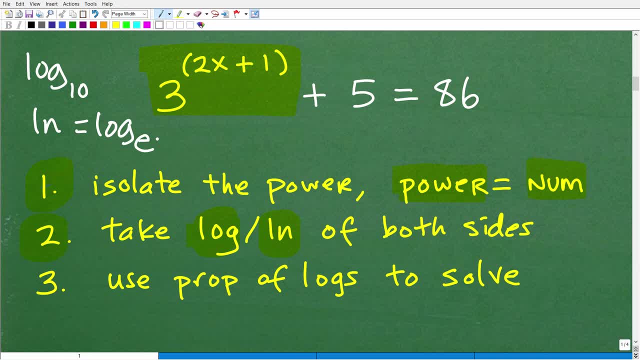 you can learn thoroughly. If you check out any one of my courses, I would recommend my algebra two course. if you happen to be in pre calculus, I teach this in that course as well, but it will not be in my algebra one course as you don't. really most students will not be able to do that. 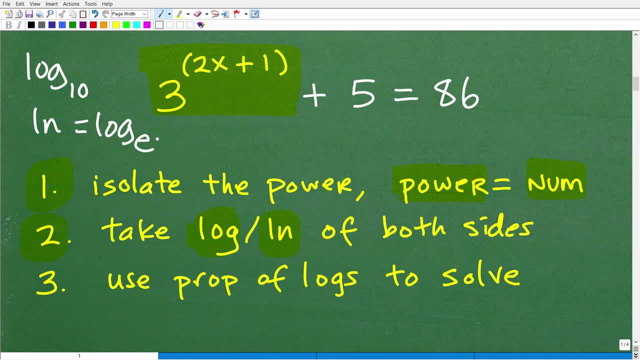 get into logarithms until algebra two or college algebra. Okay, so, anyways, we're going to go ahead and take the log of both sides. Now, how do you know whether you take the ln or common log? This is log base three. Now, if I had a problem like x or- sorry, e to the two, x is equal to one. 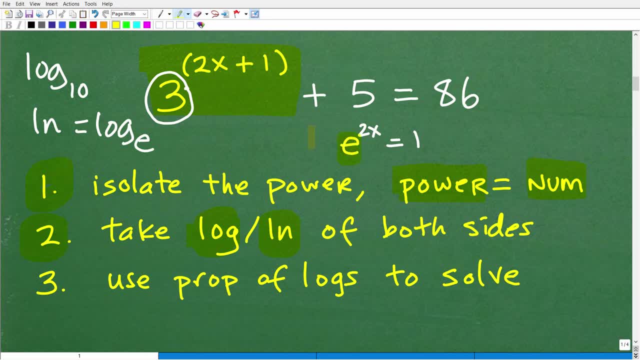 this is the natural base e. So anytime you see e, you'll take the ln, okay, the natural logarithm. If you see numbers as a base other than e, just take the log or the common log. Now, if you did take the natural log, 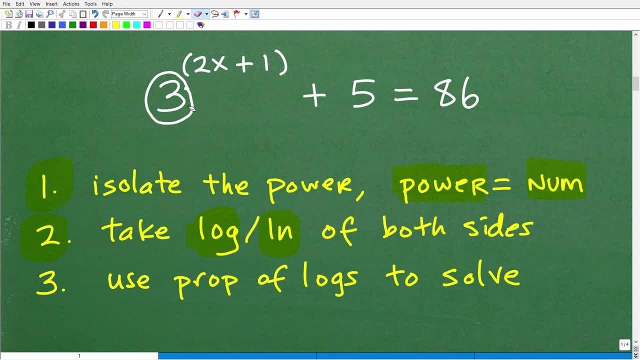 you still would get the answer right, But it's just more kind of typical to just take that common log. Okay, so we're going to take the log of both sides And then, lastly, we're going to use the property of logs, or logarithms, to solve for that variable. All right, Now, if you, you know again. 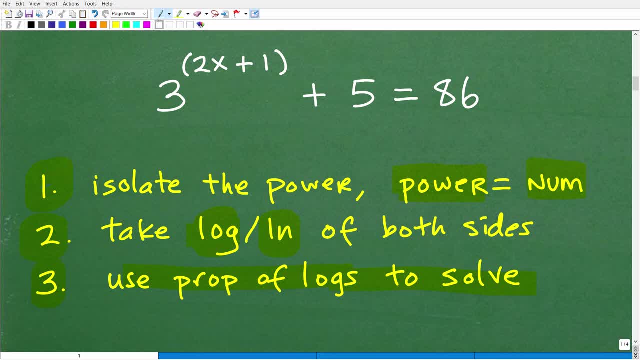 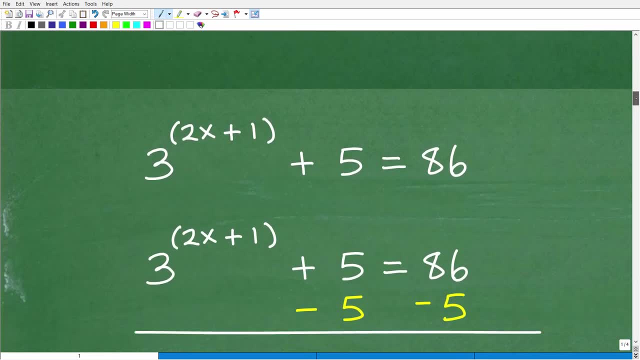 haven't studied logarithms in detail. I'm going to go ahead and show you an example of these three steps And you'll at least get a sense of what's going on. But again, if you are taking this, this should be a pretty. if you're taking algebra two or if you're studying logarithms, 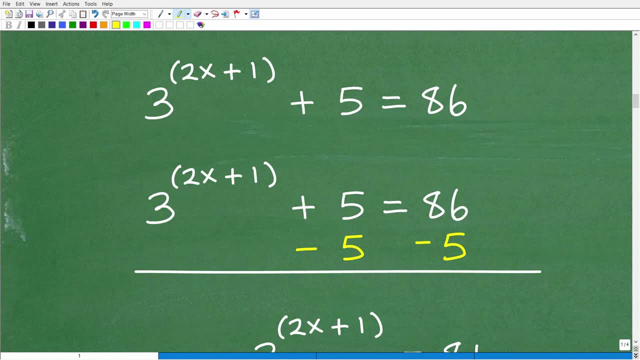 this should be a very easy problem to solve, All right, so first things first. I'm going to isolate this power, And I don't want this. I have this power plus five is equal to 86. So let's go ahead and just subtract five from both sides of the equation. In other words, I'm gonna get rid. 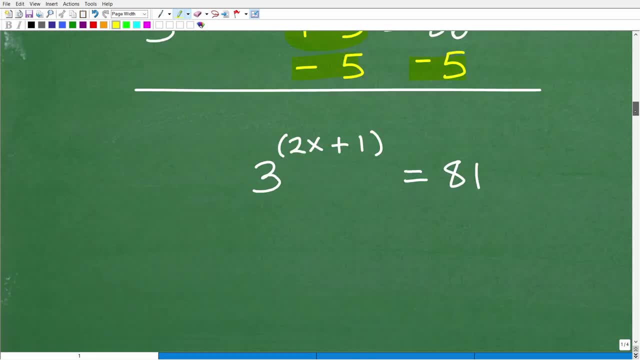 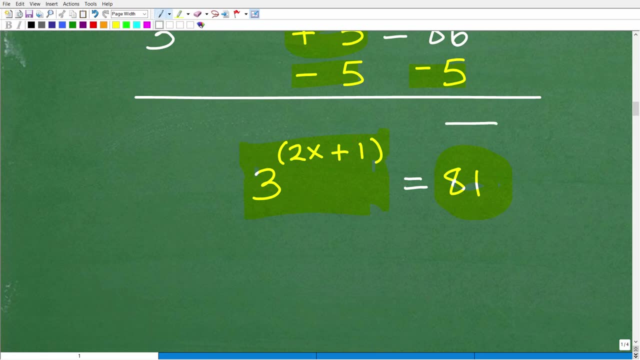 of this five, so I get the power all by itself. And when I do that, I got my power three to the two x plus one. All right, so now that is the first step. So what do I need to do? Well, now I need to take the log. 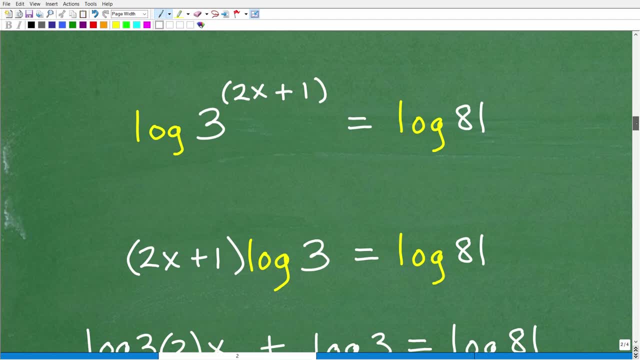 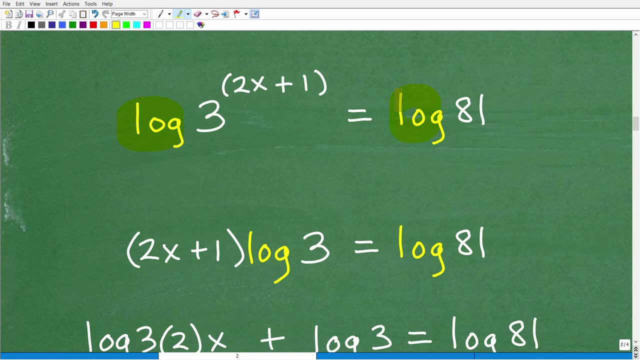 rhythm of both sides, All right, so let's go ahead and do that right now. All right, so I'm going to take the LOG of both sides and you're basically going to write it just as I'm writing right here. Okay, So one thing you need to be aware of is the logarithm of a number. okay, like the log of 81.. 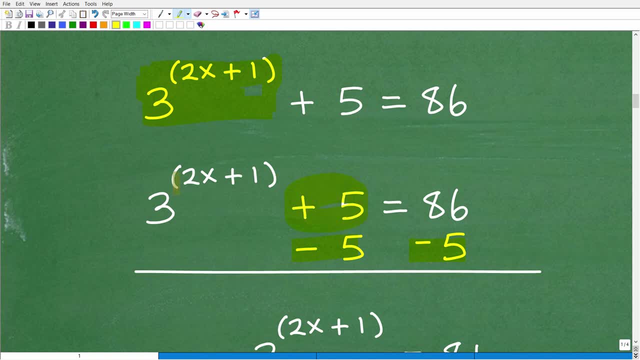 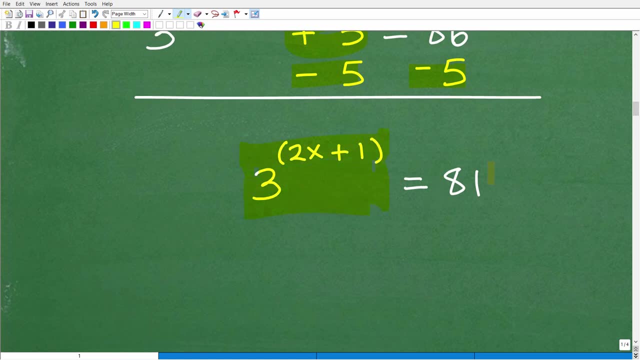 subtract five from both sides of the equation. In other words, I'm gonna get rid of this five so I get the power all by itself, And when I do that, I got my power. three to the two x plus one is equal to 81.. All right, so now, that is the first step. So what do I need to do? Well, now I 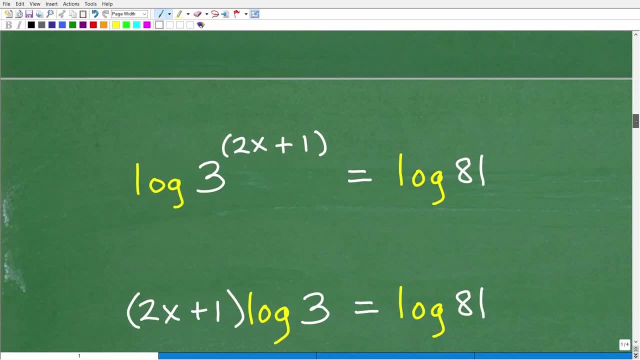 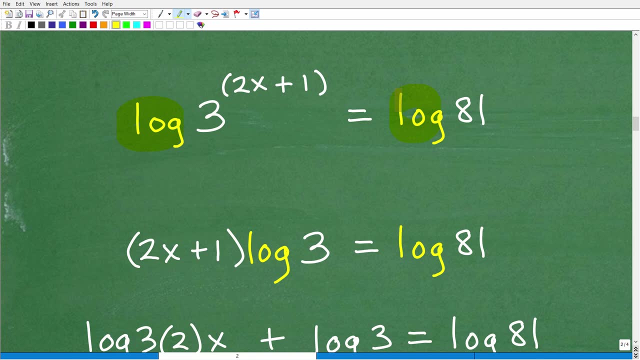 need to take the logarithm of both sides, All right, so let's go ahead and do that right now. All right, so I'm going to take the LOG of both sides and you're basically going to write it just as I'm writing right here, Okay, So one thing you need to be aware of is the logarithm of a 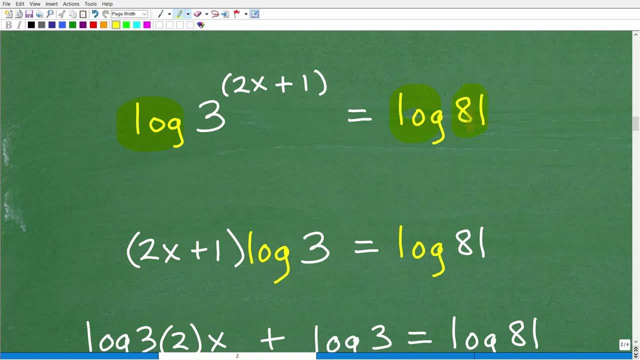 number. okay, like the log of 81.. Right, here you can. actually this is a decimal. Okay, Now you can actually compute this in your calculator. So when you're looking at this in your kind of mind's eye, just think, oh, this is just a number, right, Even though you're using 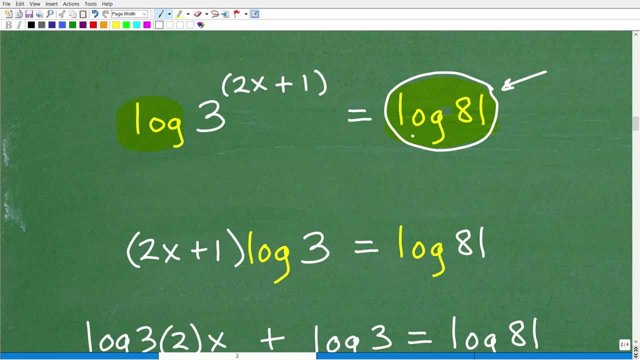 this notation LOG, you have to conceptually think of it as a number, because that's what it is. So just keep that in mind. But we're not going to actually do any number crunching right now. In other words, we're not going to convert, change this log 81 into a decimal Right now. if you've 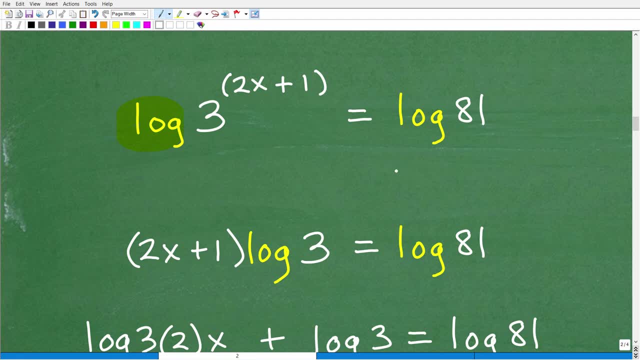 been solving your exponential equations that way. that's not a good way of doing it. We'll use our calculator at the very end of this problem. Okay, so we're taking the LOG of both sides. Now, the reason why we take the LOG of both sides is because we have a property of logarithms. It's 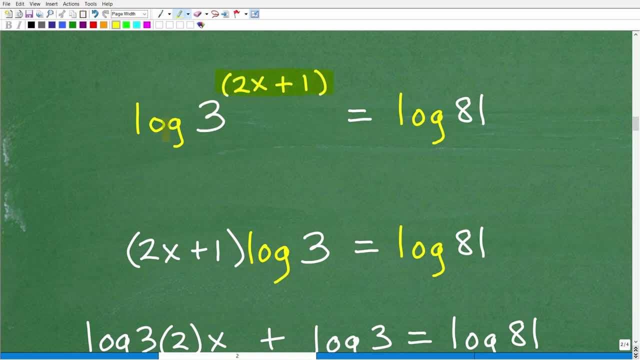 such an awesome property. Basically, what it allows us to do is, when we have a power like this and we have the exponent, when we take the LOG, we have a property that we could just take this whole exponent and put it in front of the LOG. Let me just tell you right here: if I have 2x like so, 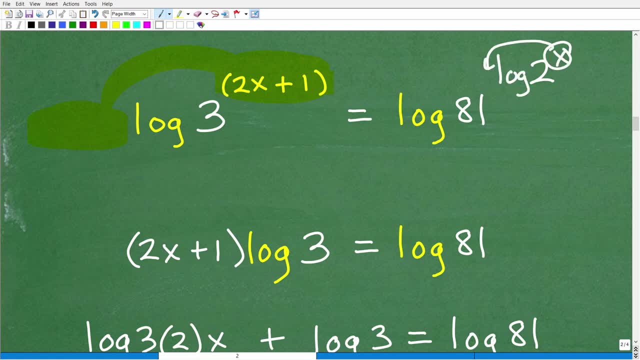 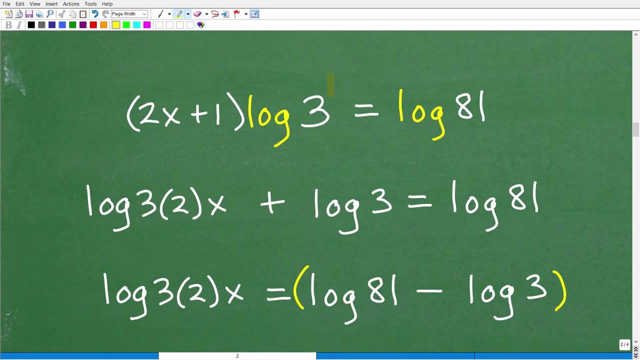 and I go LOG 2x, I can drop this x in front of the LOG. That's equal to x, LOG 2.. Okay, this is really the key to solving exponential equations: this particular LOG property. And so when we do this, we're going to end up with this right here. Okay, so notice our exponent: drop down right here. 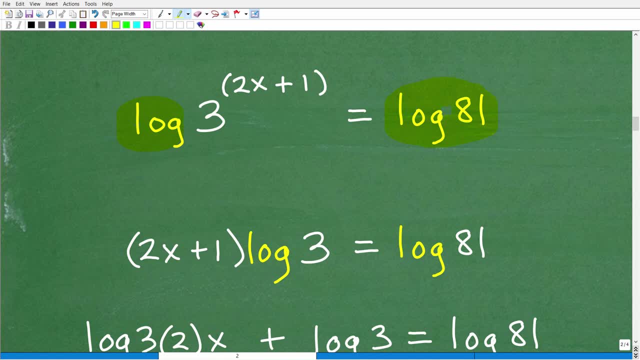 Right, here you can. actually this is a decimal. okay, Now you can actually compute this in your calculator. So when you're looking at this in your kind of mind's eye, just think, oh, this is just a number, right, Even though you're using 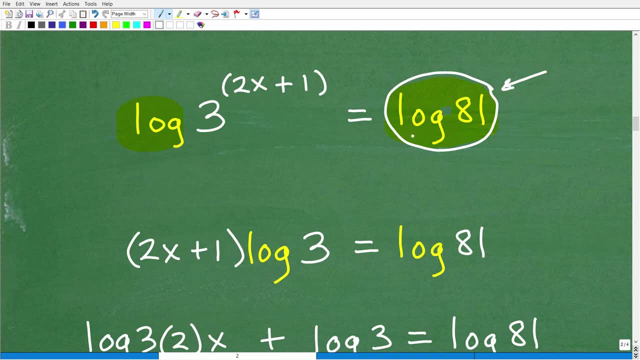 this notation LOG, you have to conceptually think of it as a number, because that's what it is. So just keep that in mind. But we're not going to actually do any number crunching right now. In other words, we're not going to convert, change this log 81 into a decimal Right now. if you've 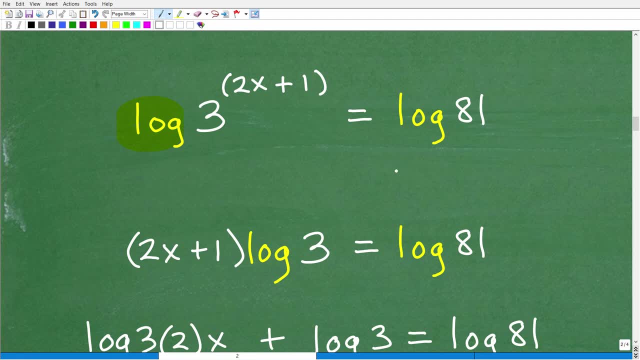 been solving your exponential equations that way. that's not a good way of doing it. We'll use our calculator at the very end of this problem. Okay, so we're taking the LOG of both sides. Now, the reason why we take the LOG of both sides is because we have a property of logarithms. It's 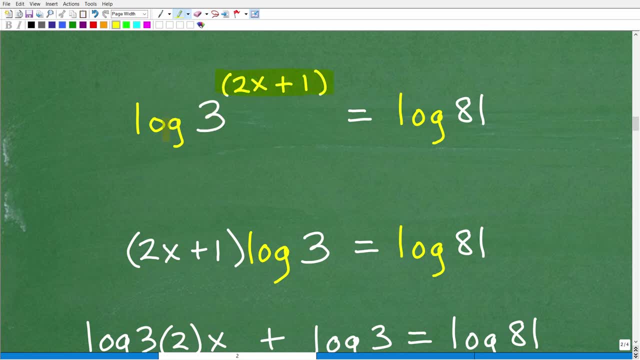 such an awesome property. Basically, what it allows us to do is, when we have a power like this and we have the exponent, when we take the LOG, we have a property that we could just take this whole exponent and put it in front of the LOG. Let me just tell you right here: if I have 2x like so, 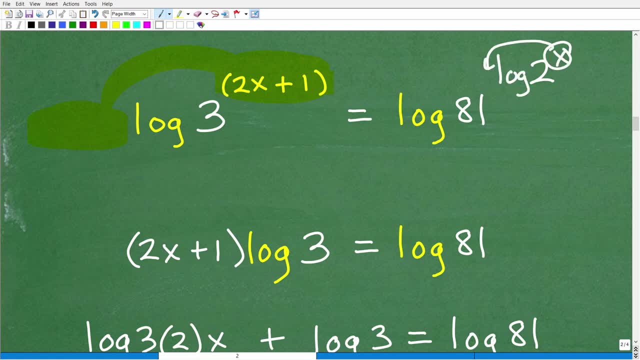 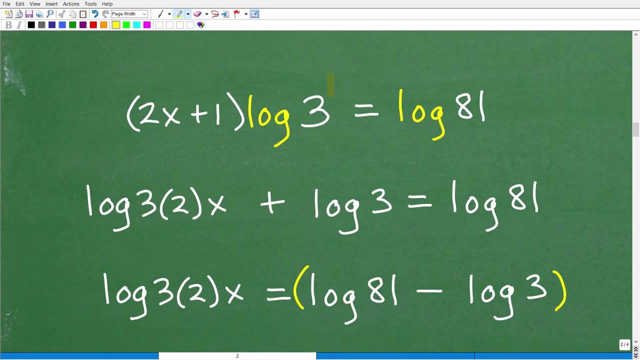 and I go LOG 2x, I can drop this x in front of the LOG. That's equal to x, LOG 2.. Okay, this is really the key to solving exponential equations: this particular LOG property. And so when we do this, we're going to end up with this right here. Okay, so notice our exponent: drop down right here. 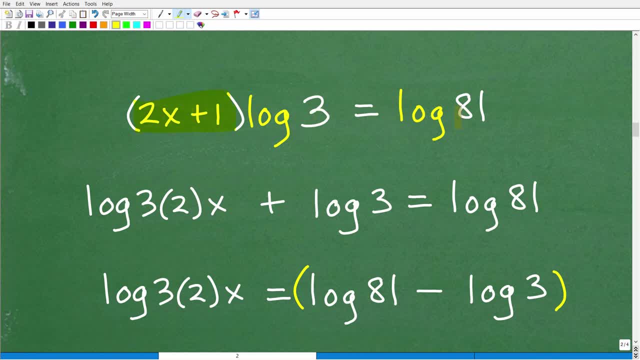 2x plus 1 times LOG 3 is equal to LOG 81.. Now, this is just a basic algebra problem. Okay, you might be saying: what are you talking about, Mr YouTube Math Man? Listen, this is a basic algebra problem because LOG 3 is just a decimal. You can convert this into a. 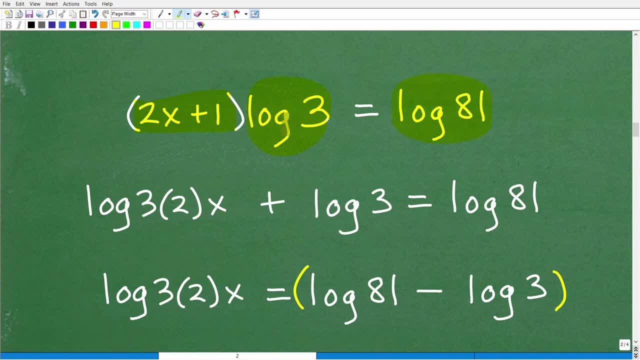 decimal right now, Same thing with LOG 81, and then just use the distributive property and your basic algebra skills to solve this equation. But you don't want to do that again right now. You want to use your calculator at the very, very end, because sometimes you're going to be given. 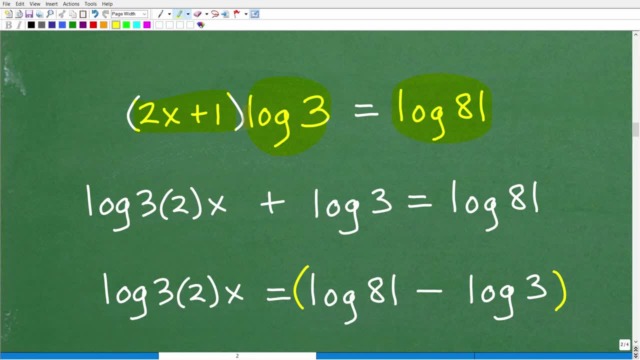 problems that you won't be allowed to use your calculator, but you can still express the final answer here without a calculator. I'll show you what I'm talking about in a second. So, but you have to keep in mind again that this is a number and this is a number. So what do we have to do? Well, we have to use the distributive. 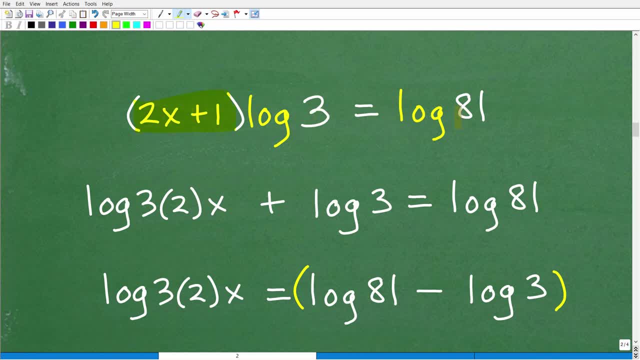 2x plus 1 times LOG 3 is equal to LOG 81.. Now, this is just a basic algebra problem. Okay, you might be saying: what are you talking about, Mr YouTube Math Man? Listen, this is a basic algebra problem because LOG 3 is just a decimal. You can convert this into a. 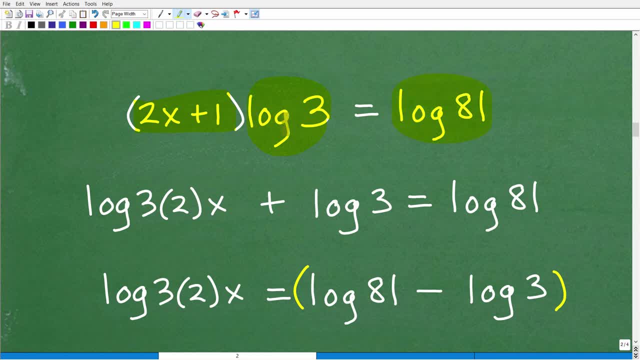 decimal right now, Same thing with LOG 81, and then just use the distributive property and your basic algebra skills to solve this equation. But you don't want to do that again right now. You want to use your calculator at the very, very end, because sometimes you're going to be given. 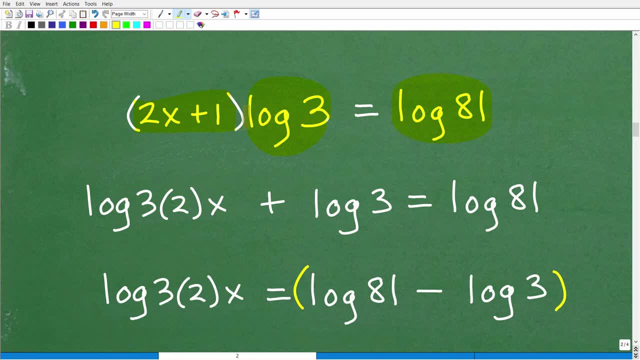 problems that you won't be allowed to use your calculator. but you can still express the final answer here without a calculator. I'll show you what I'm talking about in a second, But you have to keep in mind again that this is a number and this is a number. So what do we have to do? Well, we have to use the. 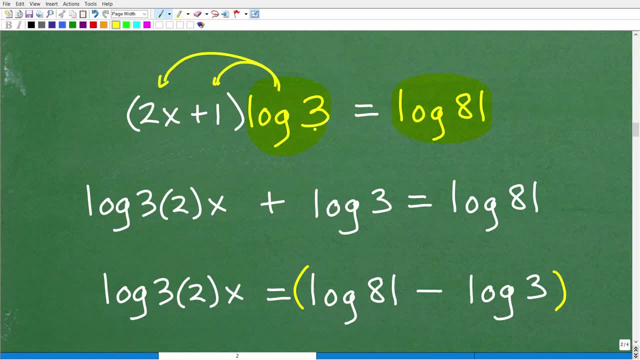 distributive property to solve for x. All right, so I'm just going to distribute this number times 2x and 1.. So that'll be LOG 3 times 2x. Now it's very tempting to take that LOG 3 and this be like: 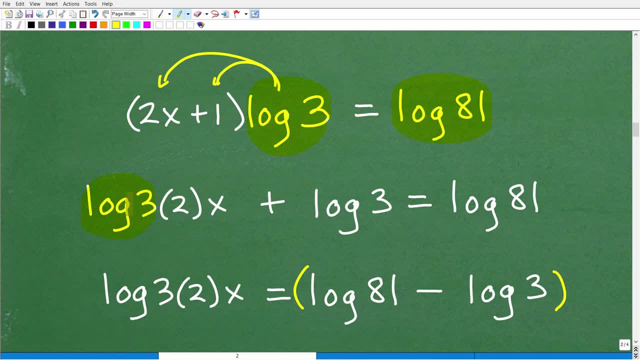 3 times 2 is 6.. You can't do that because LOG 3 is a decimal value. Okay, it's a, it's a, it's its own kind of number in and of itself. But we're going to have to figure this out in, you know. 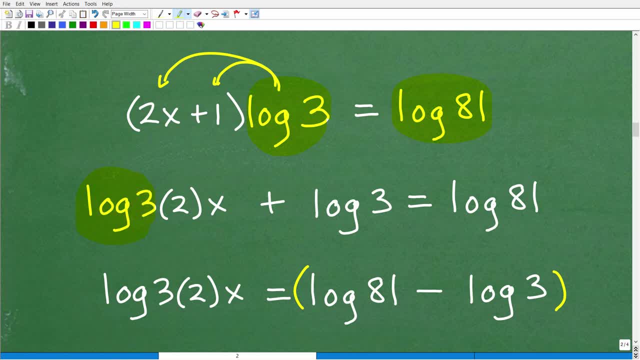 at the very end of this problem. So we're going to take LOG 3, whatever that is. then we can multiply it by 2, and that's x plus that LOG 3 times 1, and that's equal to LOG 81.. All right, 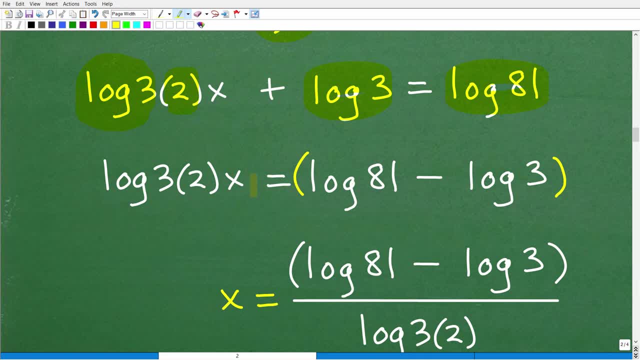 so what do we have to do? Well, just basic algebra, right? I want to solve for x, so I'm going to go ahead and subtract this LOG 3 from both sides of the equation. So that's going to give me LOG 81 minus LOG 3 again. 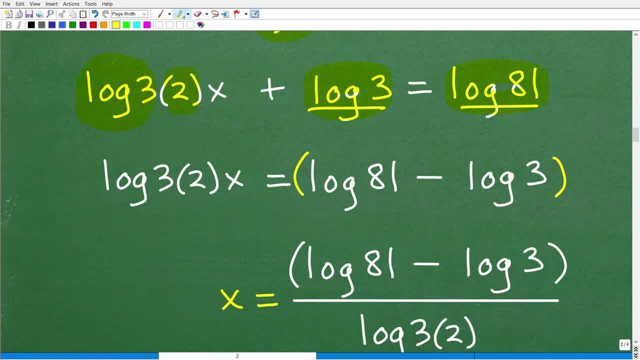 If you're confused here, just remember these are just basic. think of them as basic numbers and you'll see the steps here, right, All right, so we have. excuse me, we have LOG 81 minus LOG 3 right here, And I'm putting some parentheses in there just to kind of keep that nice and tidy. 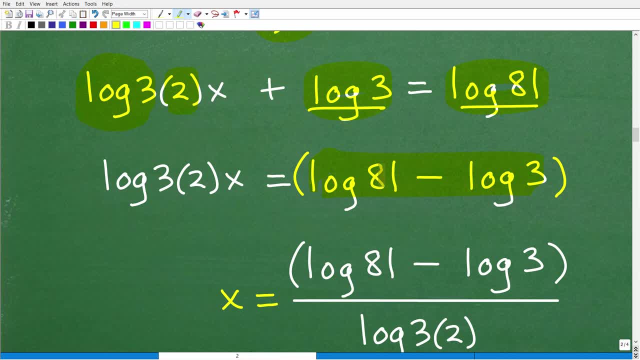 You know you should never feel shy about using grouping symbols when you're doing mathematics, okay, So you know. if you're like, do I have to put parentheses in? No, you don't have to, but it's a good idea, especially when you're dealing with sums and differences. All right, 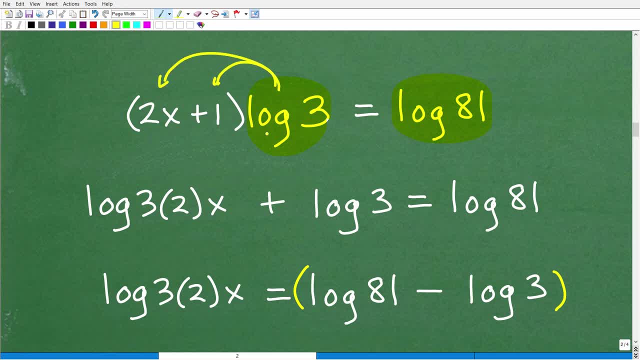 property to solve for x. All right, so I'm just going to distribute this number times 2x and 1.. So that'll be LOG 3 times 2x. Now it's very tempting to take that LOG 3 and this be like: 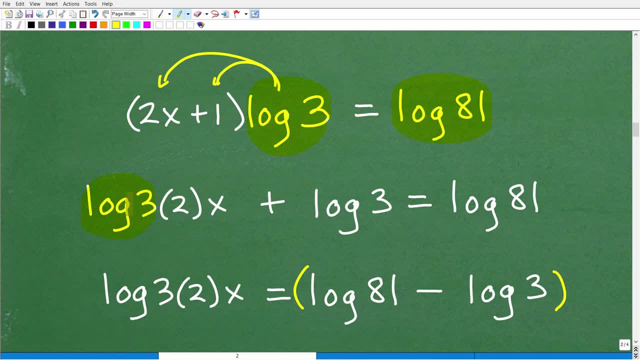 3 times 2 is 6.. You can't do that because LOG 3 is a decimal value. Okay, it's a, it's a, it's its own kind of number in and of itself. But we're going to have to figure this out in, you know. 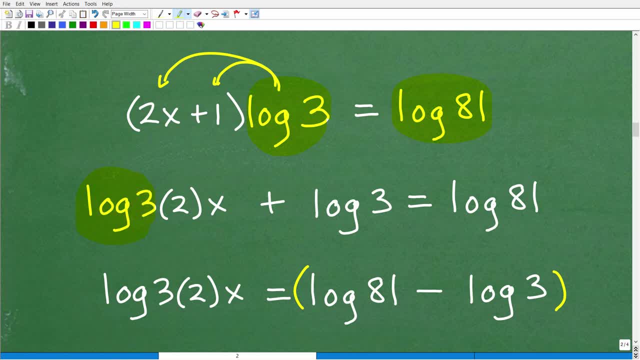 at the very end of this problem. So we're going to take LOG 3, whatever that is. then we can multiply it by 2, and that's x plus that LOG 3 times 1, and that's equal to LOG 81.. All right, 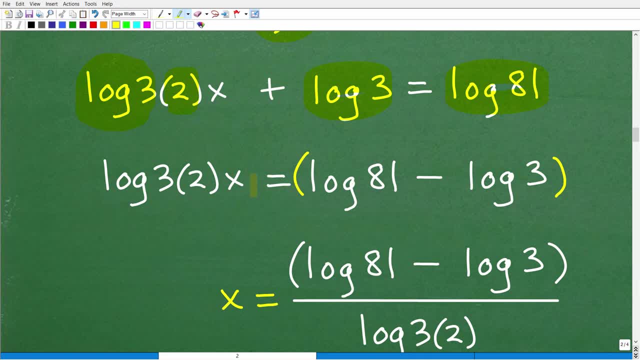 so what do we have to do? Well, just basic algebra, right? I want to solve for x, so I'm going to go ahead and subtract this LOG 3 from both sides of the equation. So that's going to give me LOG 81 minus LOG 3 again. 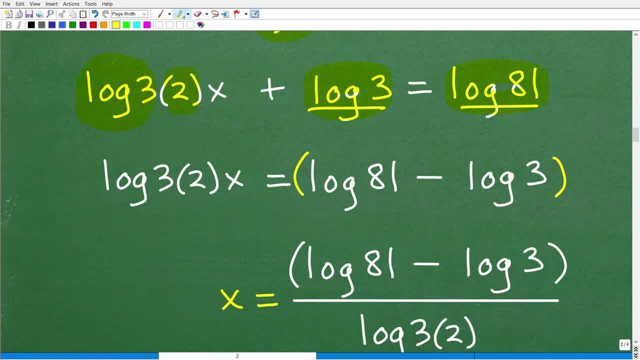 If you're confused here, just remember these are just basic. think of them as basic numbers and you'll see the steps here, right, All right, so we have. excuse me, we have LOG 81 minus LOG 3 right here and I'm putting some parentheses in there just to kind of keep that nice and tidy. 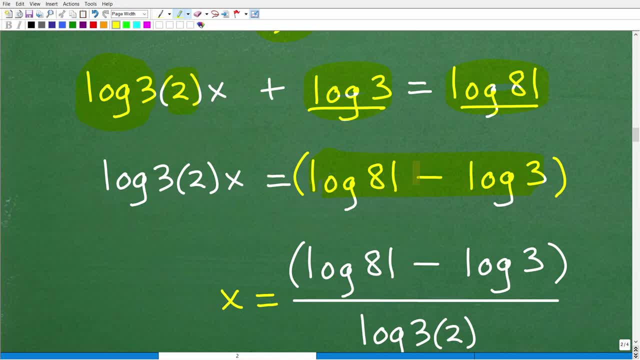 You know you should never feel shy about using grouping symbols when you're doing mathematics, okay, So you know. if you're like, do I have to put parentheses in? No, you don't have to, but it's a good idea, especially when you're dealing with sums and differences. All right, 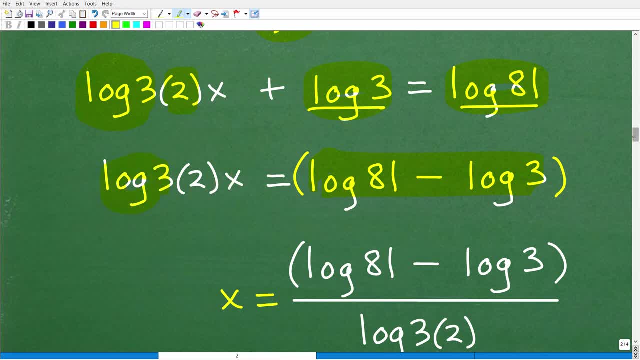 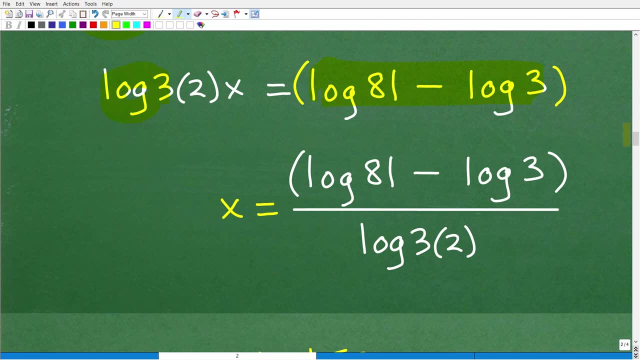 so here we have our LOG 3 times 2x, and this is where a lot of you that know what you're doing could get in trouble if you know, because you're kind of just you know doing the algebra here. 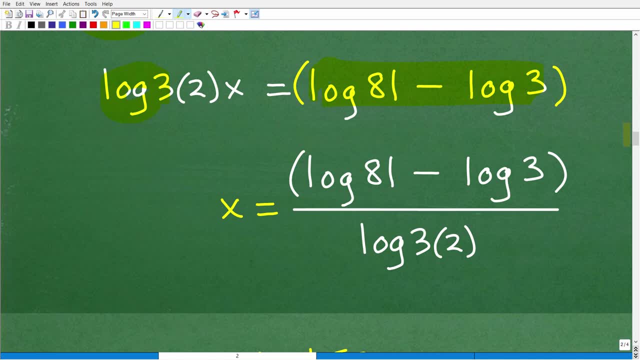 and you have to really pay attention that you're not, you know, writing anything incorrectly. So the final answer for x is what? Well, this is just a number, so I need to divide both sides of the equation by this number. so we have LOG 81 minus LOG 3, all that divided by LOG 3 times 2.. So now, 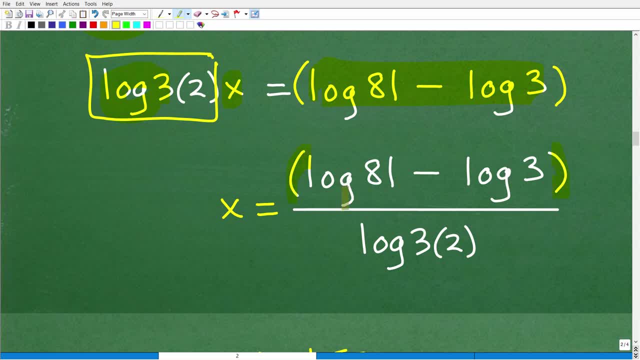 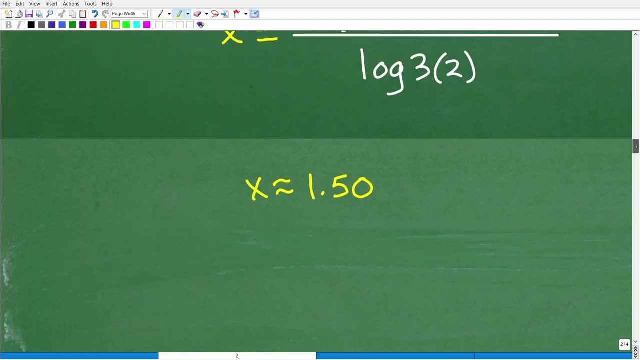 you have to get your calculator and you have to divide both sides of the equation by this number. you have to get your calculator out and use parentheses if you're not comfortable typing all this in at one shot into your calculator. the answer again is going to be 1.5, approximately 1.50. 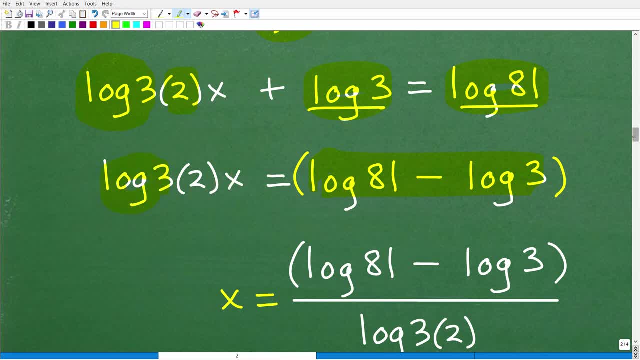 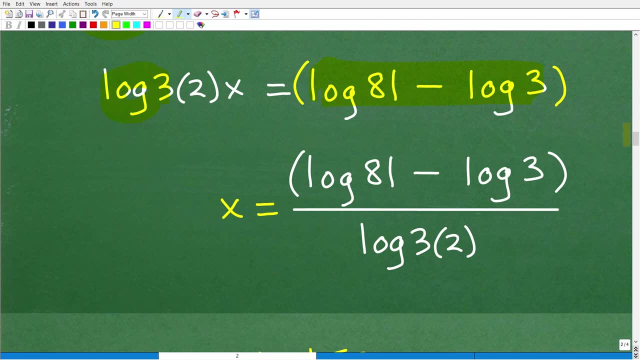 so here we have our LOG 3 times 2x, and this is where a lot of you that know what you're doing could get in trouble if you know, because you're kind of just you know doing the algebra here. 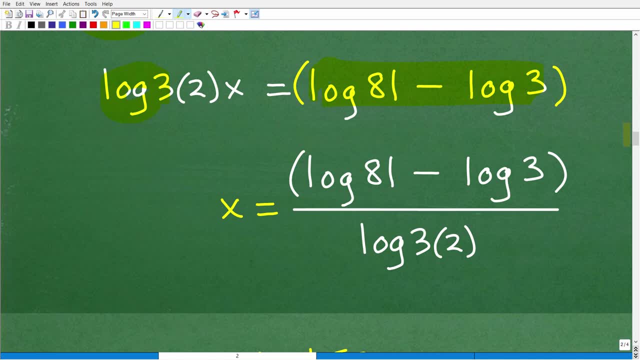 and you have to really pay attention that you're not, you know, writing anything incorrectly. So the final answer for x is what? Well, this is just a number, so I need to divide both sides of the equation by this number. So we have LOG 81 minus LOG 3, all that divided by LOG 3 times 2.. So now, 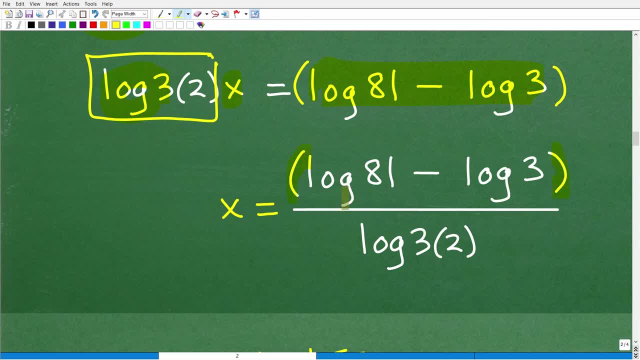 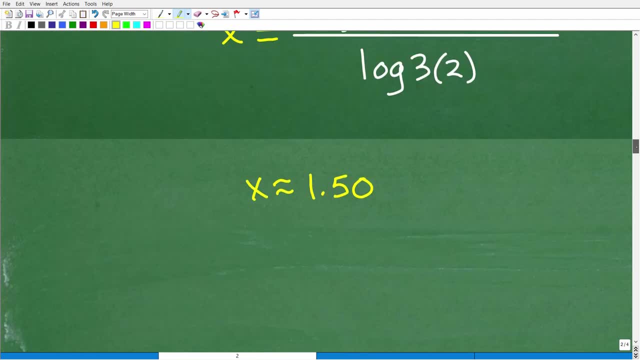 you have to get your calculator and you're going to have to divide both sides of the equation by. you have to get your calculator out and use parentheses If you're not comfortable typing all this in at one shot into your calculator. the answer again is going to be 1.5, approximately. 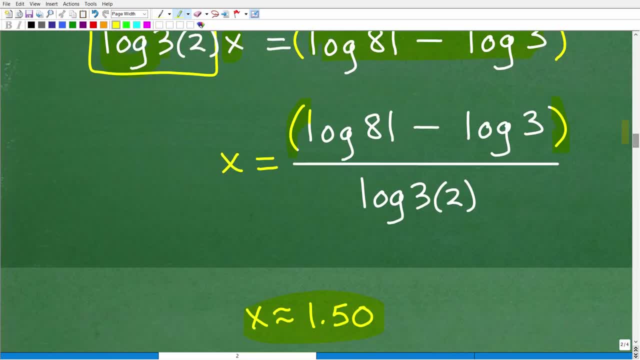 1.50.. So go ahead and practice doing this Now. if you're like, oh, you know, this is a lot to kind of type in at once, Well, what you can do is just type: get this, get the answer to this. 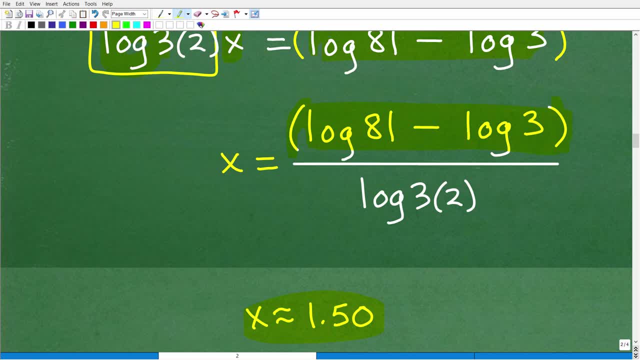 LOG 81 minus LOG 3, get that decimal value and then divide it by LOG 3.. You have to find the LOG 3 first and then multiply it by 2, and then just take these two numbers and divide them. 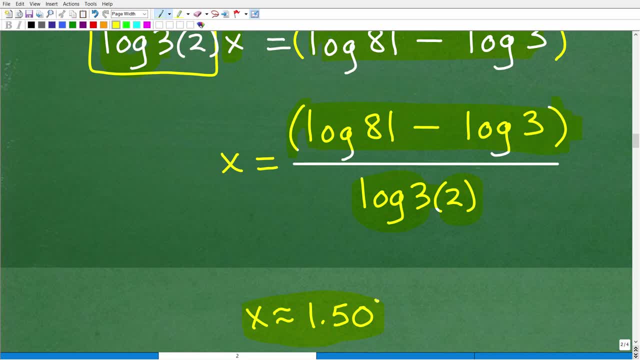 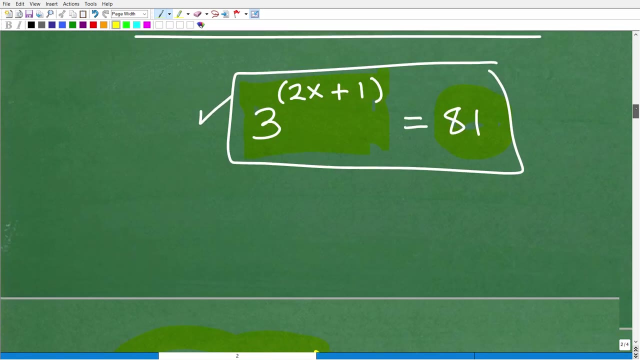 and you should get approximately 1.50.. Now I'm going to strongly suggest that if you are at this particular level of mathematics- Algebra 2, College Algebra Pre-Calculus- that you get really good at using your graphing calculator or scientific calculator For most. 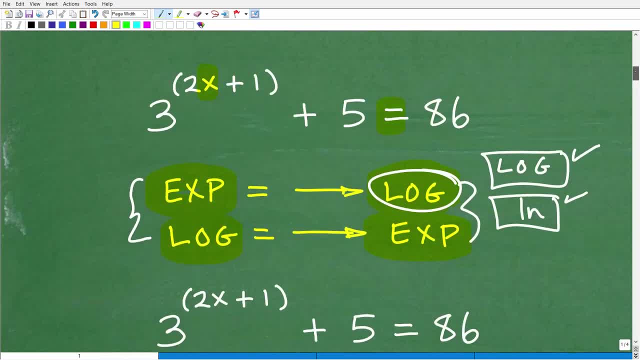 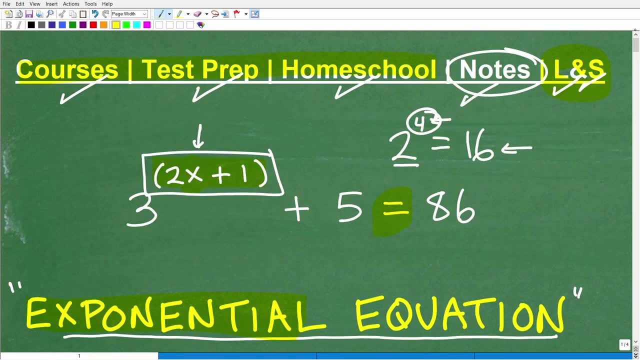 of you out there, it will be a graphing calculator and that's better because the graphing calculator has a bigger value. So if you're at this particular level of mathematics- Algebra 2, College Algebra, Pre-Calculus screen, so you can see what's going on. But in terms of exponential equations, I would say 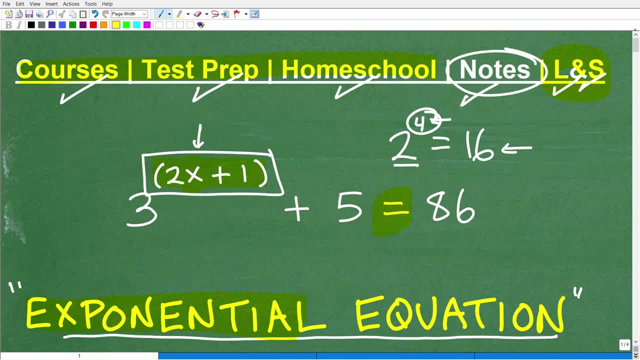 that you know it's kind of like your salsa or hot sauce, right, You have like the mild, the medium and then the hot. This problem here was, I would you know classify as kind of like a mild. It's not that difficult of a problem in terms of exponential equations. So if you found 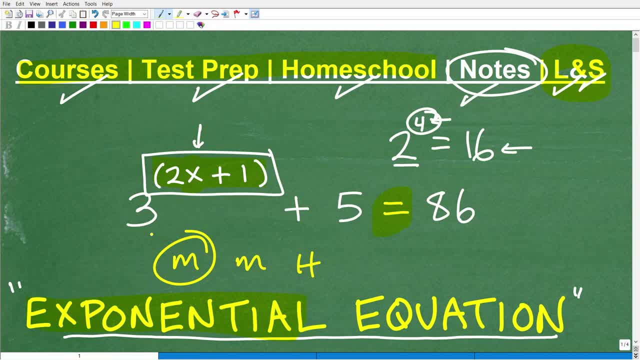 this difficult. you just simply need to learn you know, learn the material, the topics involved, the skills involved, and practice, practice, practice And make sure you can do these more advanced level problems Okay. So, with that being said, 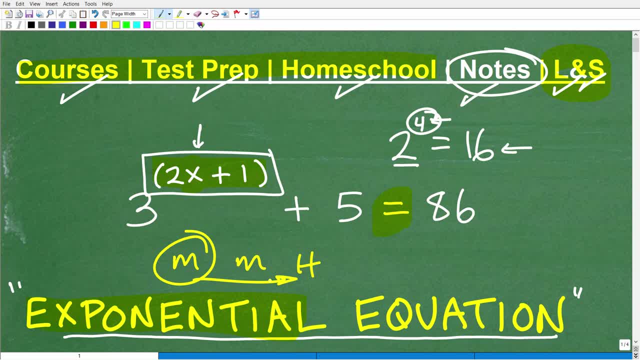 I definitely wish you all the best in your mathematics adventures. Thank you for your time and have a great day.